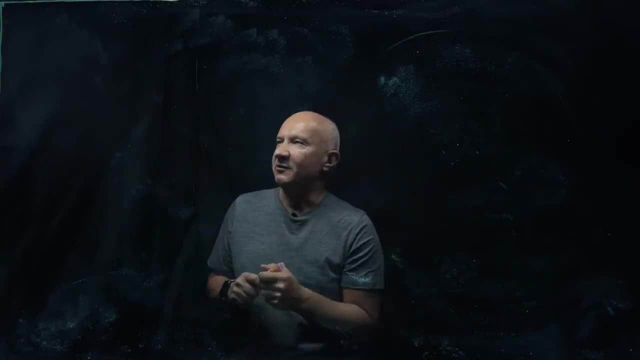 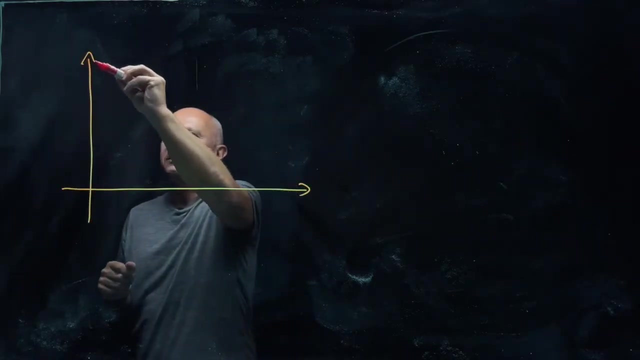 a lot of problems. We all do, of course, but you know they can also quantify it. So what they do? if they want to quantify problems into those two classes, easy or difficult- they look at the scaling, So they pick up an algorithm for a given problem and then 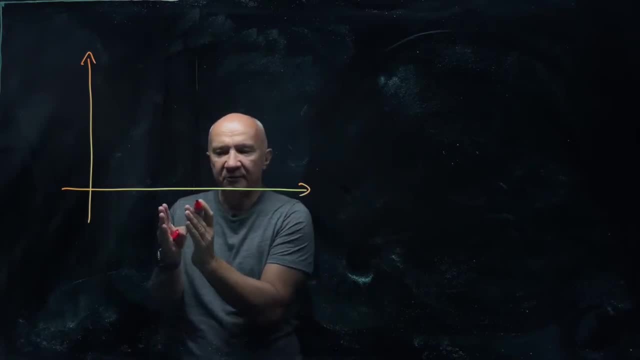 they apply this algorithm, try to solve the problem for increasing size of the input. So, for example, take multiplication. that's your problem. You have a good algorithm for multiplication, So what do you do? You apply this algorithm to one-digit number, then you multiply it to two-digit number, to three-digit number. 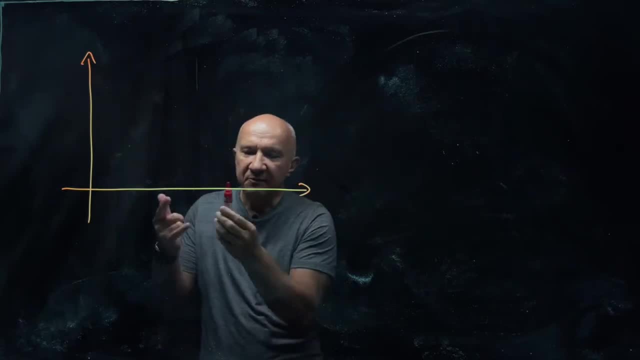 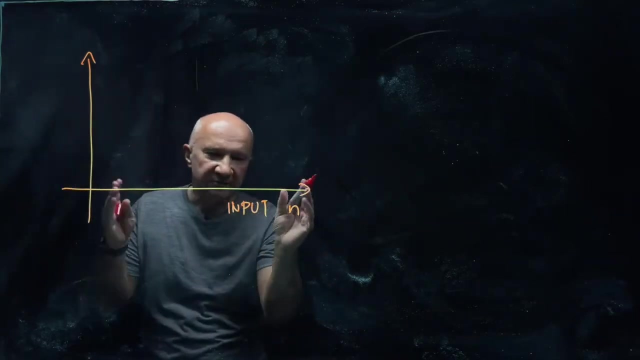 and so on and so forth. So you put the size of the input as the number of digits. You put it on the horizontal axis, So let's call it input, So n is the number of digits. And then you look at the execution time, So of course it grows as you increase the size of 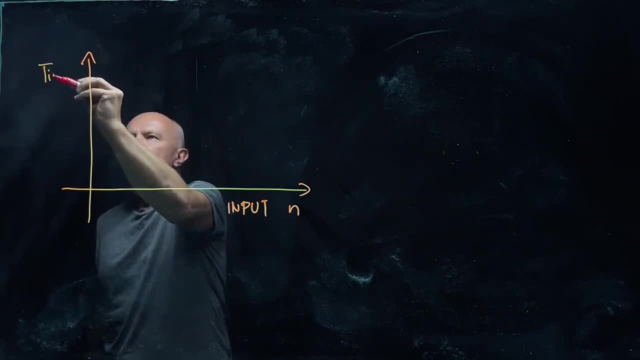 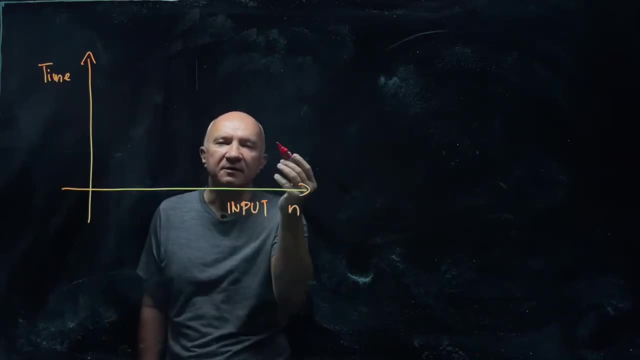 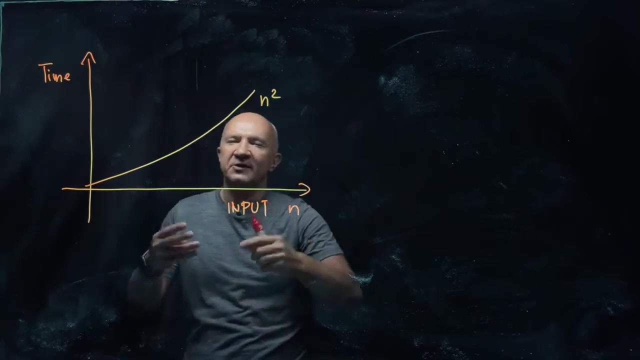 the input And on the vertical axis you have this execution time. Now when it gets bigger it grows like logarithmic, linear at most, polynomial function of the size of the input, say n squared. Then computer scientists say, well, great, fantastic, this is a good algorithm. 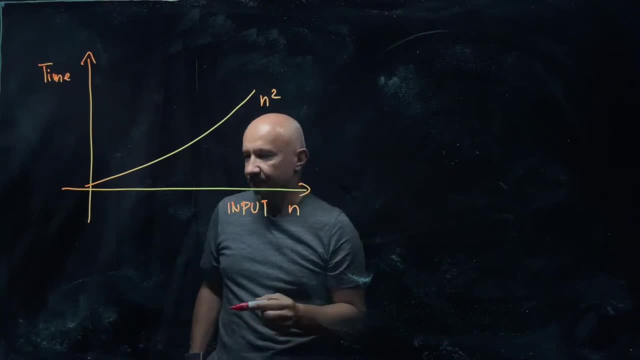 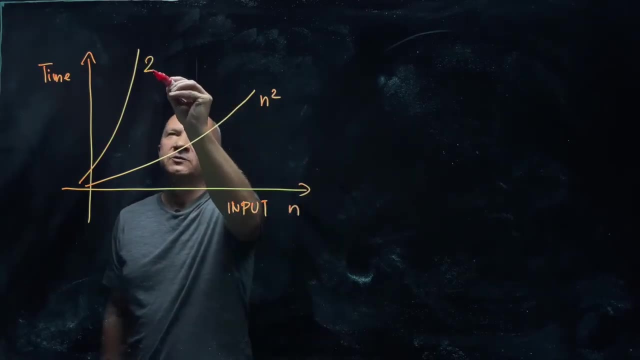 The execution time doesn't grow too fast, We can handle it. However, whenever it goes as the exponential function of the size of the input say two to the n, then computer scientists are not happy. They say: well, we know how to solve the problem, but let's. 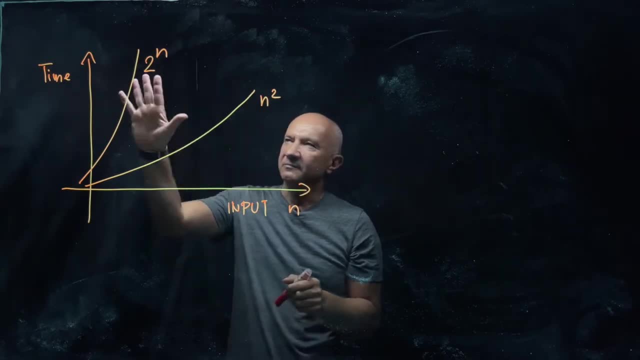 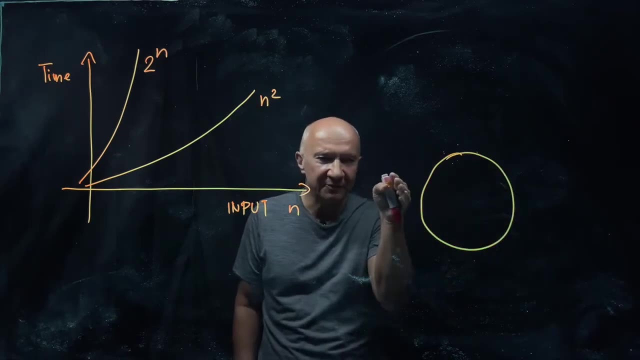 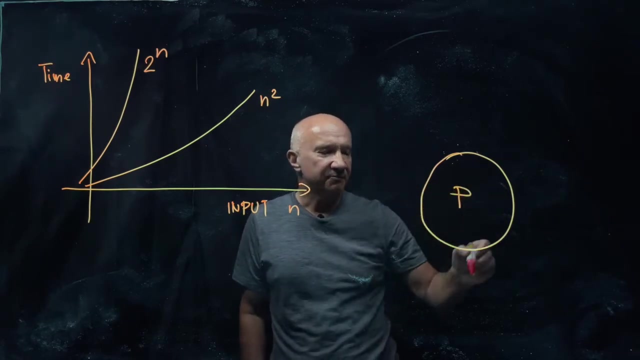 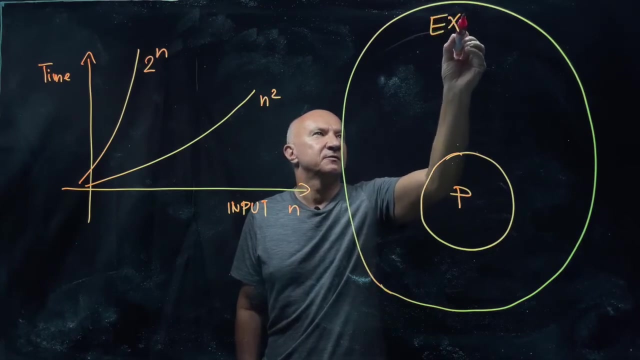 see if there's another efficient way of solving the problem. And then they just draw complexity classes. They say, OK, all problems that we can solve on a deterministic classical computer in polynomial time, call this class p. Then of course this is a subset of a huge class of problems that require exponential time to solve them. Now 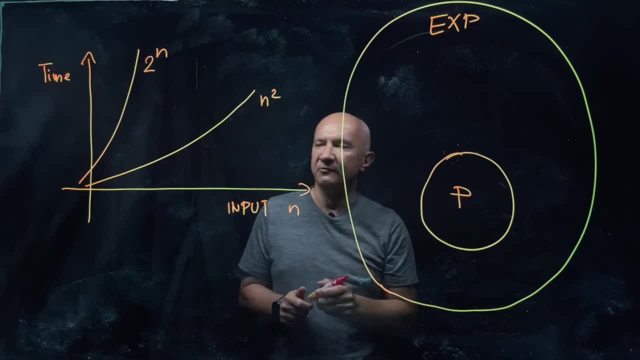 then we look at, say, probabilistic model of complexity And we look at random computation And we ask questions: OK, well, how about randomized computation? when you use randomness as an extra resource for computation, Then computer scientists think, well, maybe, maybe that they give us some advantage, Maybe the class? 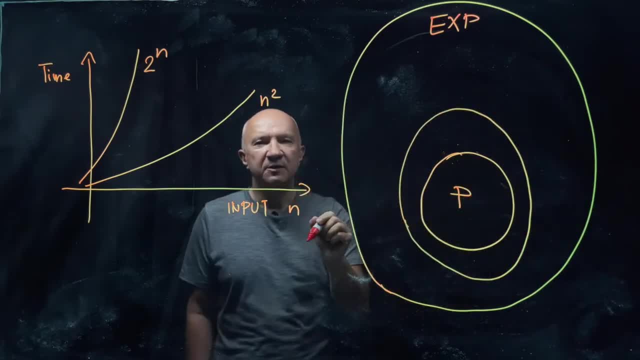 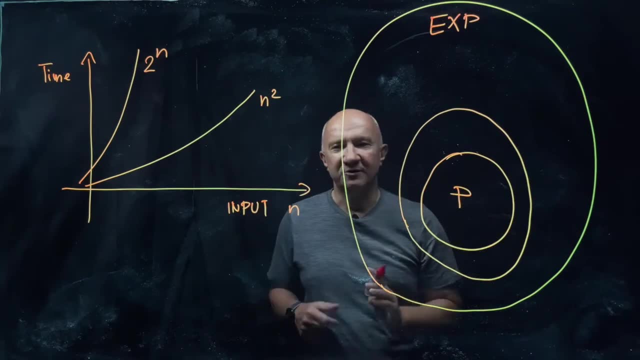 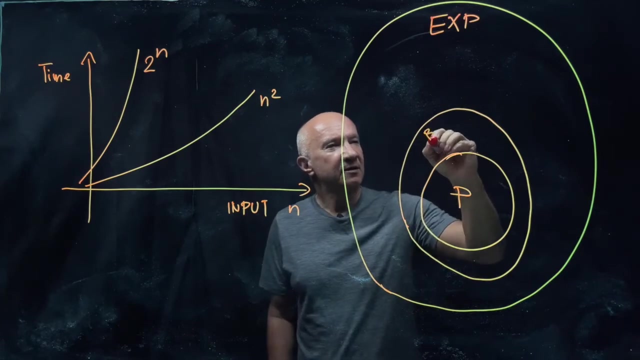 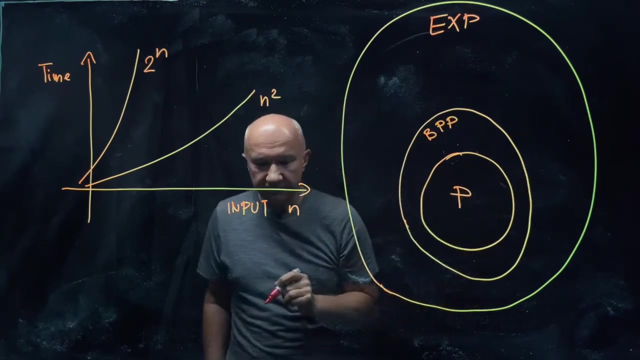 of problems that can be solved in polynomial time on a probabilistic computer is slightly larger. That's actually not known. Many things in computational complexities are essentially not known, But the class that is called BPP, that stands for bounded error, probabilistic polynomial. 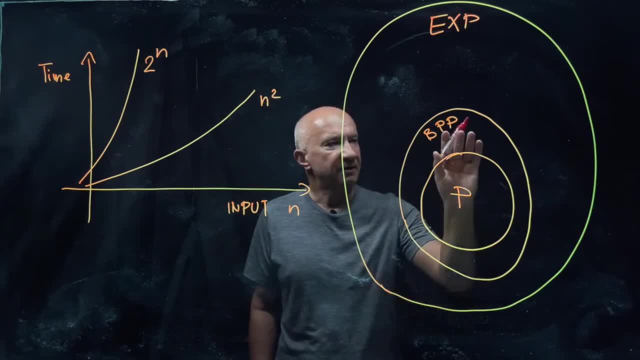 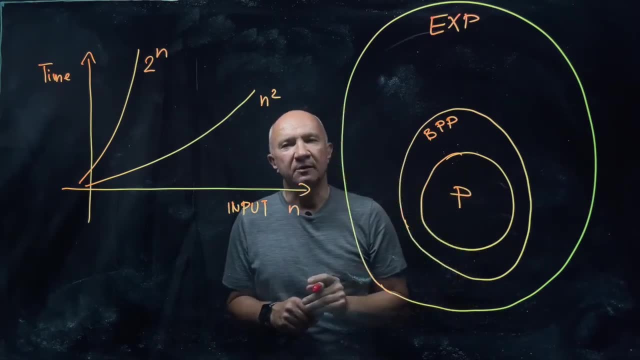 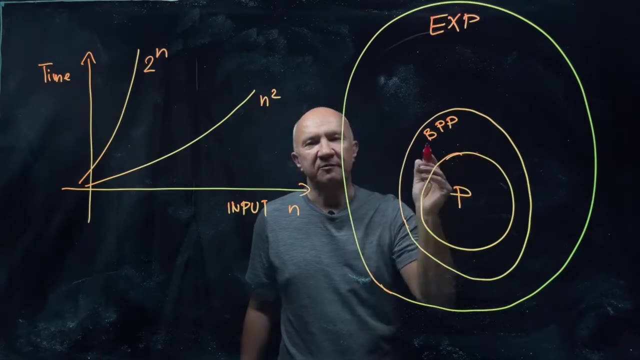 may contain problems that can be solved in polynomial time using randomness, But we don't know how to solve them on a deterministic classical computer in polynomial time. Over time there was, you know there were a few problems. If I were Giving these lectures many years ago, I would probably 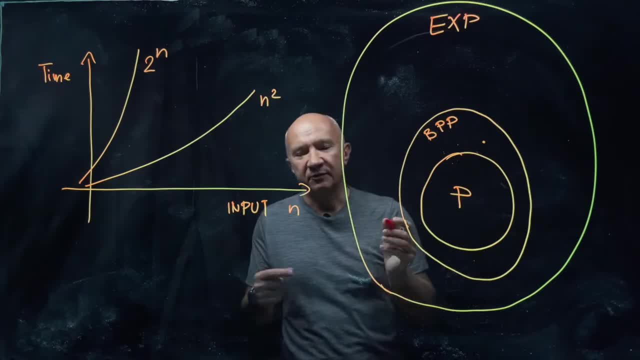 tell you that there is a problem that is here, for example, testing whether a given number is prime. But over time people found a deterministic algorithm, so the testing whether a given number is prime is now in p. So there is a remarkable migration of problems from 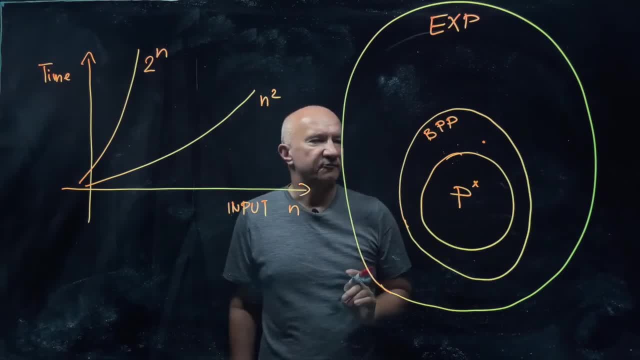 BPP to p, but still we don't know whether those two classes are different or the same. So it could be that BPP is equal to p. Nobody knows at this point. What we are interested in is another class is a class of. 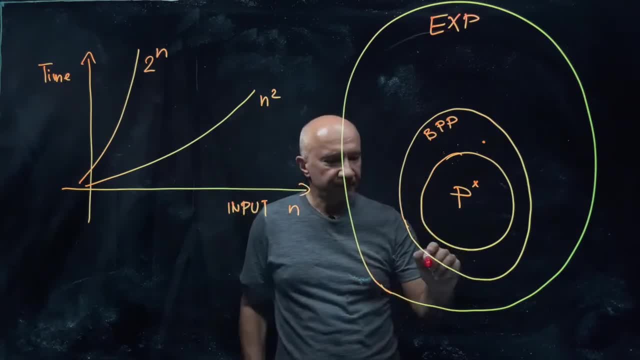 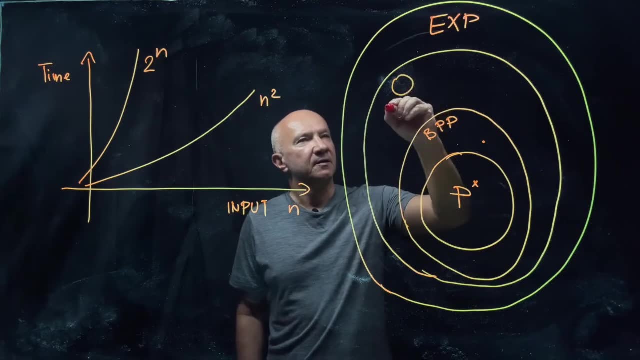 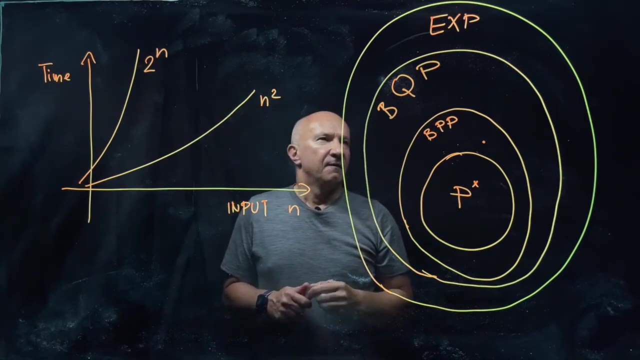 problems that quantum computers can solve in polynomial time, And this class is larger than BPP, So we call it BQP, That would be bounded-arrow, quantum polynomial time. There are problems in this class, for example factoring of large integers. 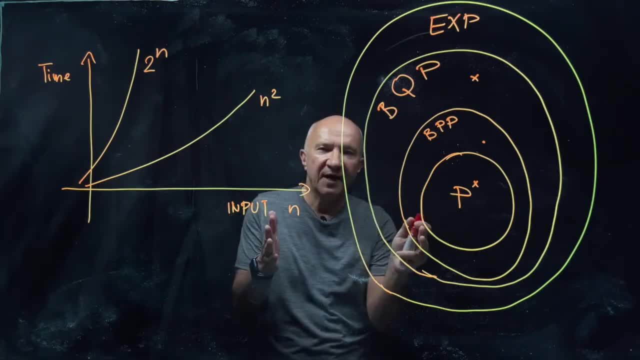 So if we want to decompose a given number into prime factors and if we increase the size of the number, it's getting exponentially difficult to find those factors, And that is the case for any type of classical computation, be it deterministic or probabilistic. 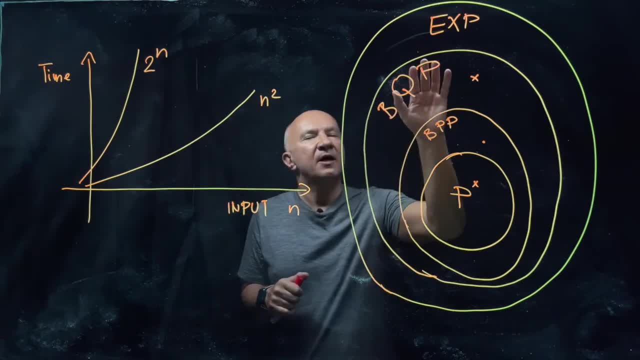 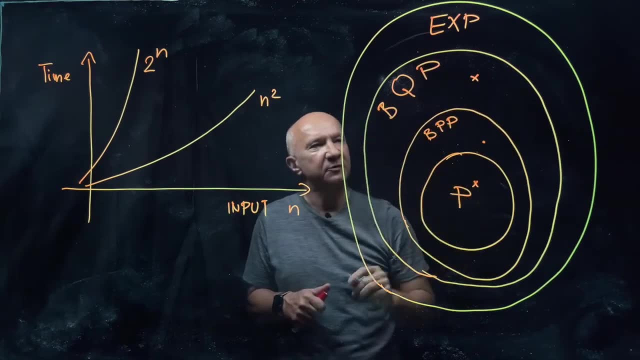 We simply don't know how to do it. Now we know how to do it with a quantum computer, So there are problems. that And that's what makes computer scientists really excited about. They find it fantastic because the way they define difficult.